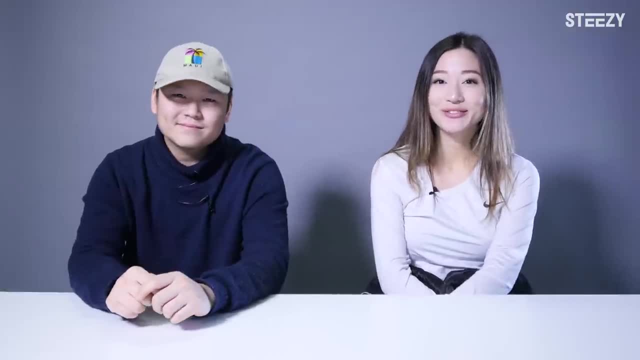 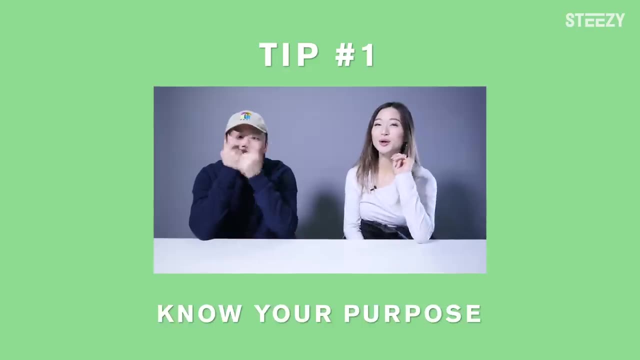 Hey guys, this is Jessie and Clay, and in this video you're going to learn how to choreograph your very own dance routine using these six easy tips. Tip number one: know your purpose, Not like in life or anything, but why are you making this dance routine in the first place? 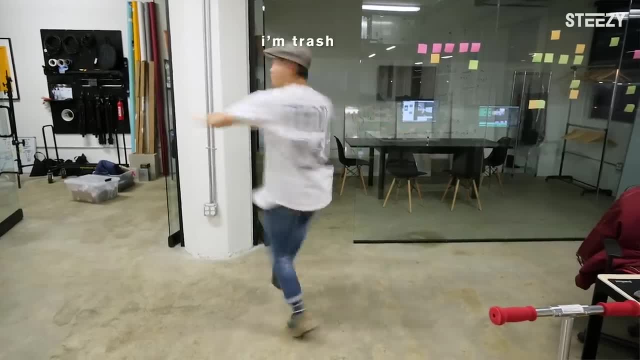 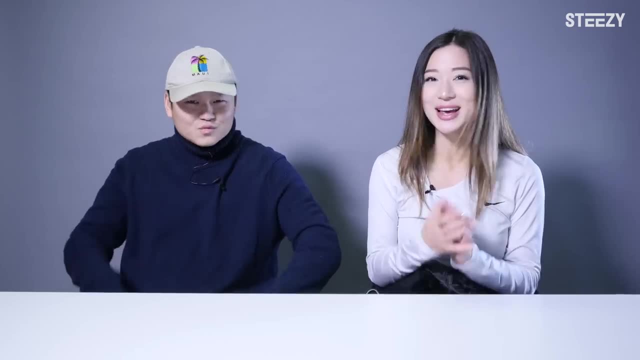 And who are you performing in front of? Are you making it for a solo ballet recital? Is it for a teen competition? Are you making a concert video for YouTube? Are you performing at your grandma's 80th birthday party? Thinking about these things will help you choose your song, the length of the piece and also the types of movements that you want to incorporate. 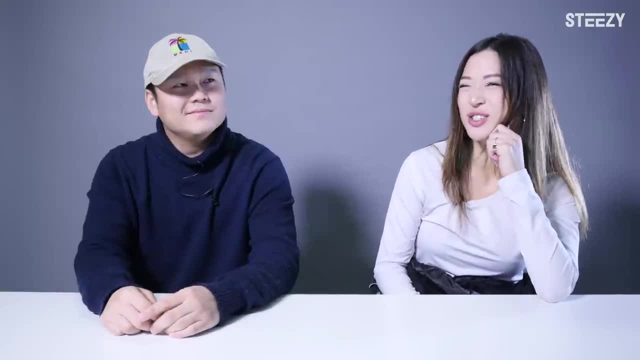 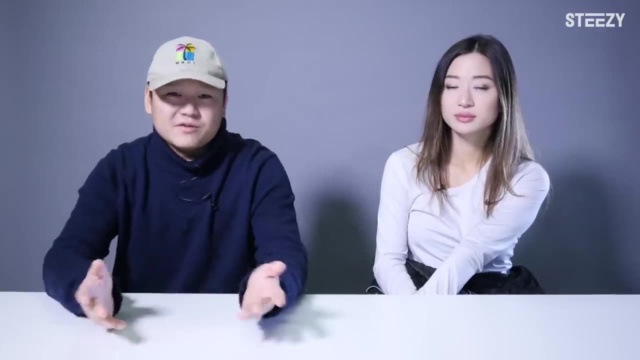 Yeah, you don't want to be twerking at your grandma's 80th birthday party, Unless she's into that. Tip number two: pick a song, cut it or mix it. You don't have to hire a DJ or anything crazy, but you just got to pick out which part of the song that you enjoy. 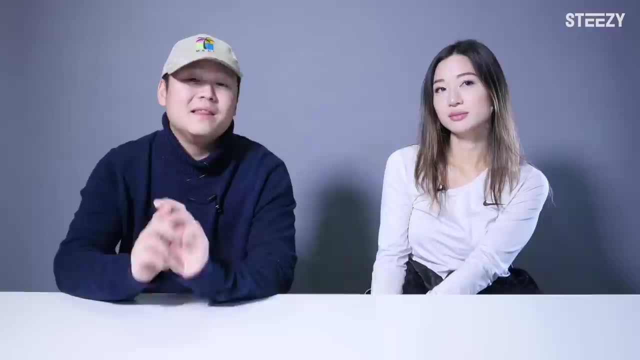 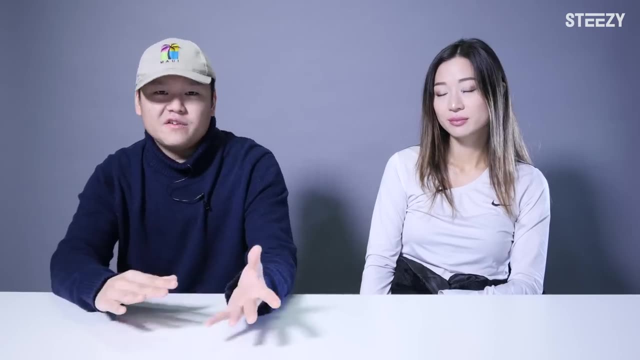 which ones that you may want to cut and bring together or just change out. This is going to help you map your piece out. Speaking of tip number three, map out your routine. Decide the major section of the choreography or moves that you want to do. 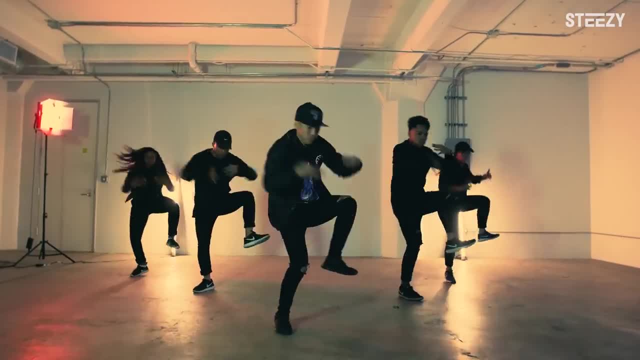 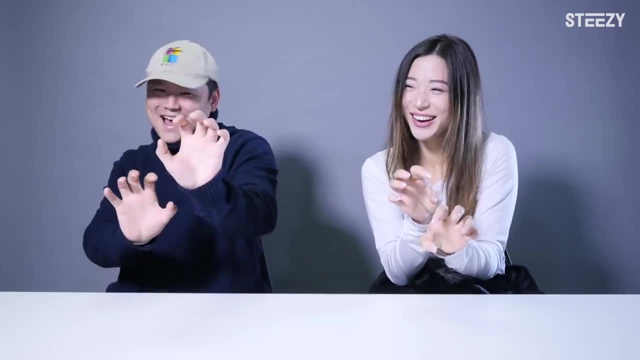 So maybe the intro starts off slow, smooth and sexy, and then the chorus gets really, really hype and then closer. you're just going to kill it off. You know, just meow, Meow, Meow, And then you can fill in those in-between sections. 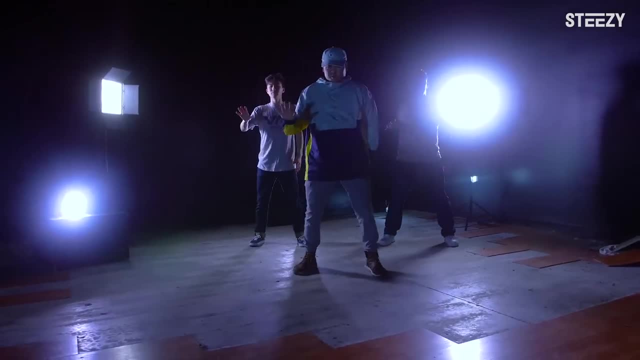 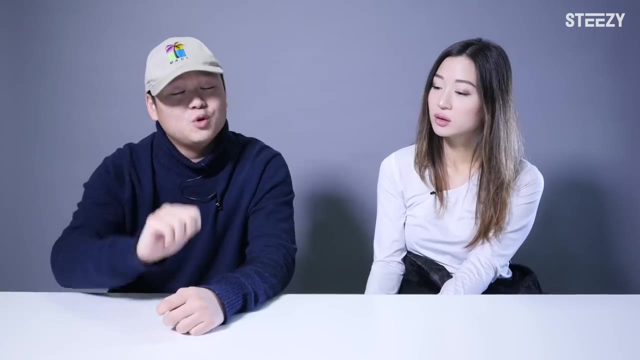 What I generally do is I'll pick out my song, pick out my favorite beats or moments sounds inside the song, and then I will freestyle and record it so that I can just watch myself later and go, ooh, that was a cool move. Then I'll keep that move and put it in my choreography. 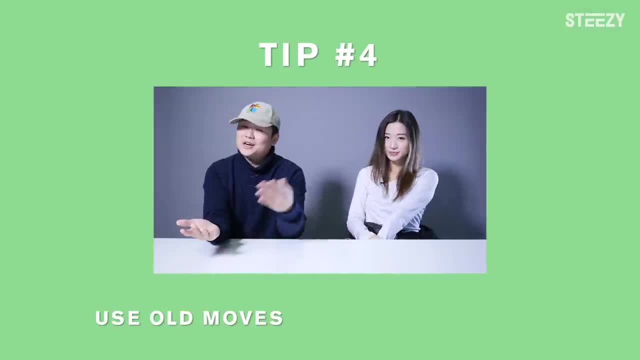 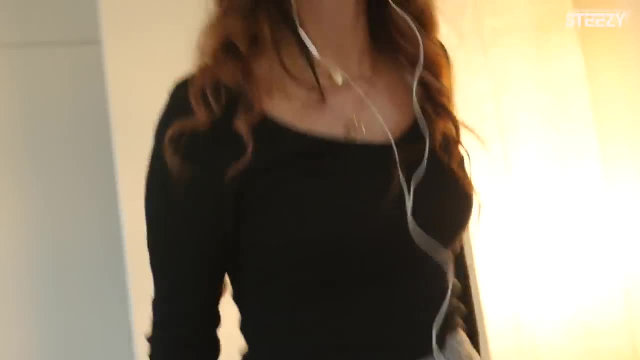 Tip number four: use some old moves And then try out some new ones. You might feel lost on how to even start choreographing a piece, because you're sitting there expecting some crazy new, unique movements to just come to you and they're not coming to you. 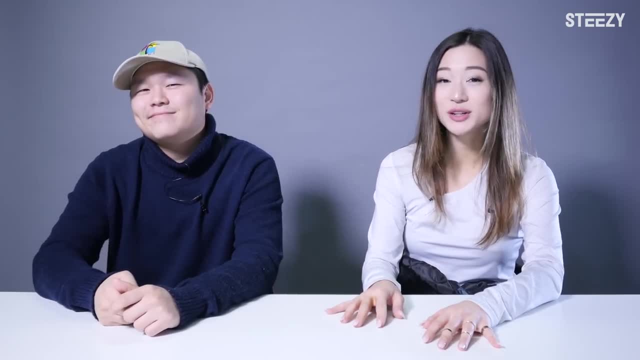 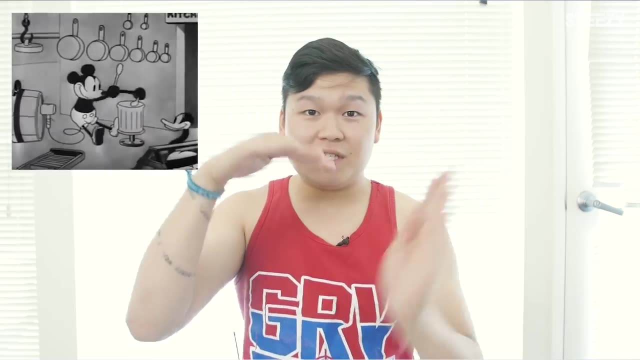 So just start by doing moves that already feel comfortable to you, and we'll explain how to spice them up a little bit later. Once you have a base of comfortable moves, then it's time to come up with some new ones. We have a whole video on how to use concepts to create moves. 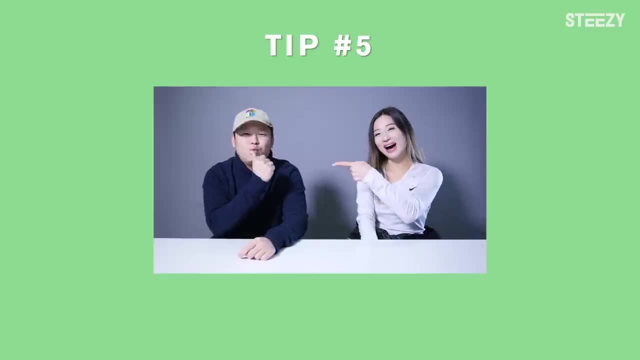 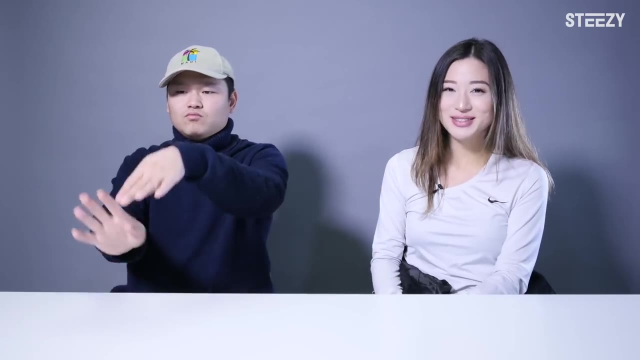 so make sure you click that link in the description to watch it. Tip number five: embellish and edit. Hmm, Okay, let's go back to your comfort moves now. You can give them a little flavor by playing with different elements in choreography.